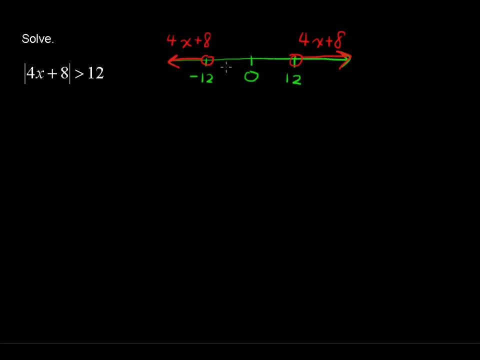 and graph that That's going to set up two inequalities. So let's write those down right. Just take it right from the graph. there You have 4x plus 8 is less than negative 12, or you have the other. 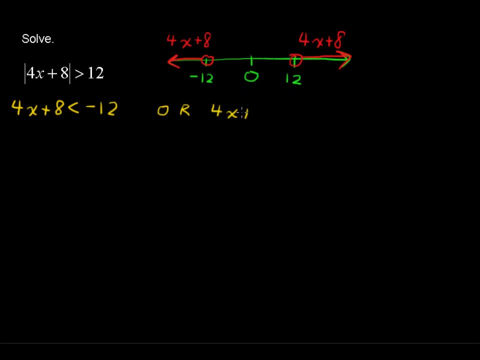 scenario where 4x plus 8 is greater than positive 12. 12 units from 0.. And yeah, this will set up two solutions, but that's okay, That's what we want. So here we're going to solve these equations. 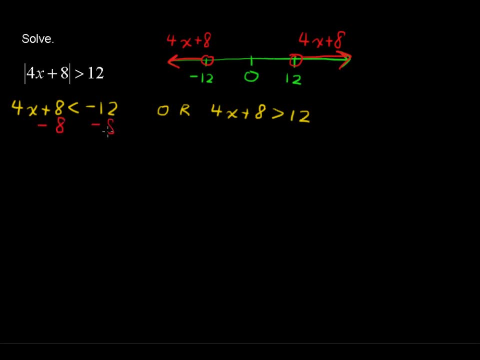 Let's subtract 8 from each side, and we can even solve these simultaneously, just because we're doing the same thing: to isolate the variable, to isolate x, And what we get on this inequality is 4x. 4x is less than. 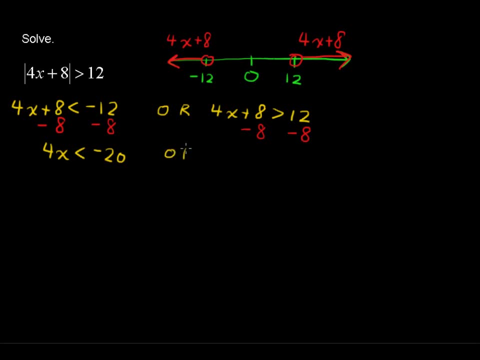 negative 20, or with our other inequality we have, 4x is greater than 4.. Our next step to isolate the variable is to divide by the coefficient, divide by 4.. So let's show that, Divide everything by 4.. 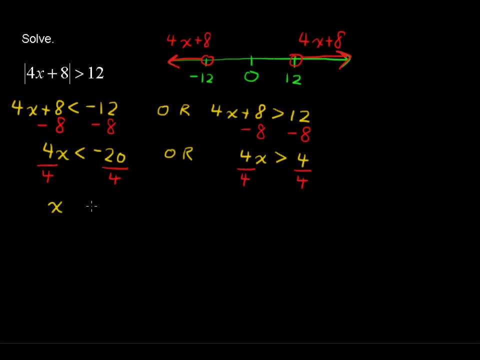 That's going to give us as a result, x is less than negative 5, or we have x is greater than 1.. So we really have this. Our solution contains these two sets of numbers. You can write this in set notation if you'd like: less than negative 5.. So set notation from: 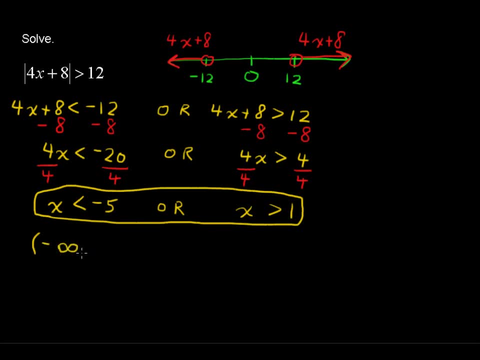 negative infinity, and you always use the rounded parentheses there for negative infinity or positive infinity Up to negative 5, rounded parentheses because it's negative, 5 is not included, or now we can say these numbers as well, greater than 1, and. 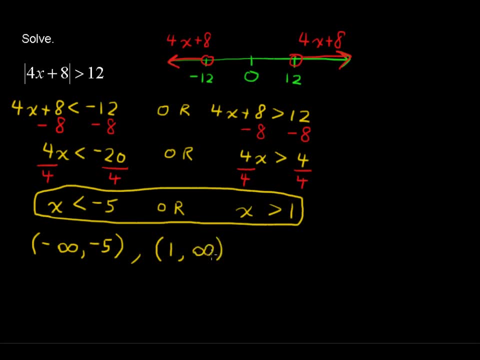 to the right: forever. Infinity is not a number, It's just an, just an idea. Goes on forever. Okay, so all of these numbers, Let's graph that. Let's graph all of these numbers so we can show visually our solutions.